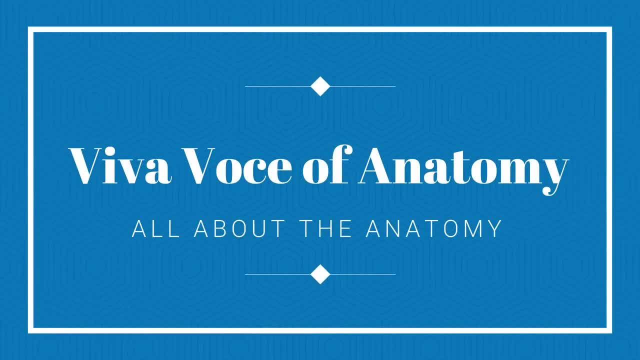 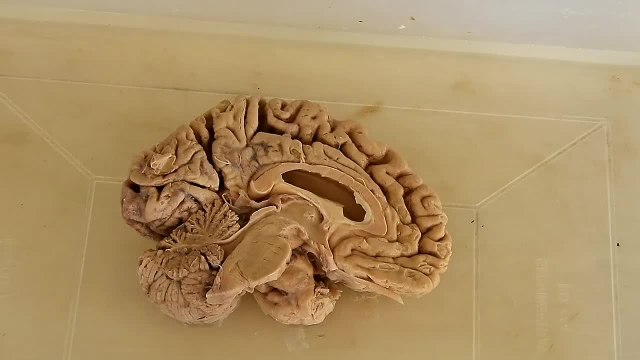 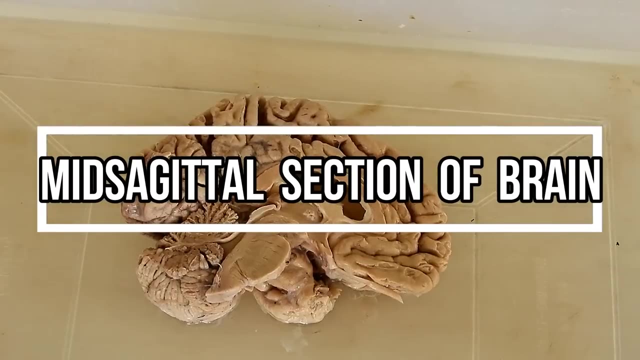 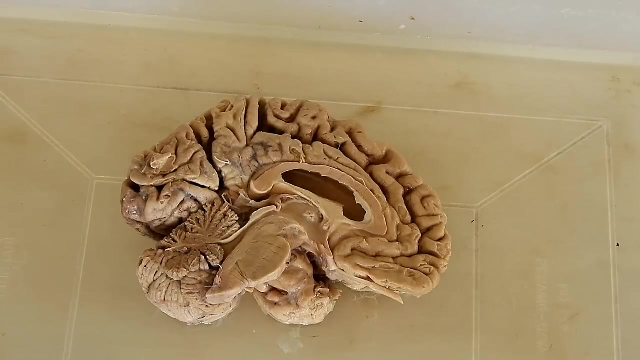 Hello friends, welcome to the Vaibhavos of Anatomy. Today we will see the medial section of a brain, But before that we will see the parts of a brain. The brain is divided mainly into three parts, That is, forebrain, midbrain and the hindbrain. Now the forebrain. 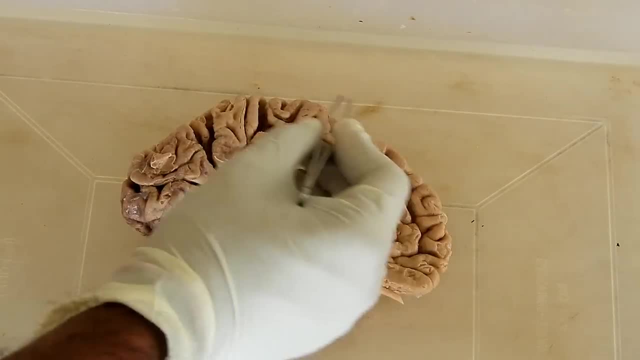 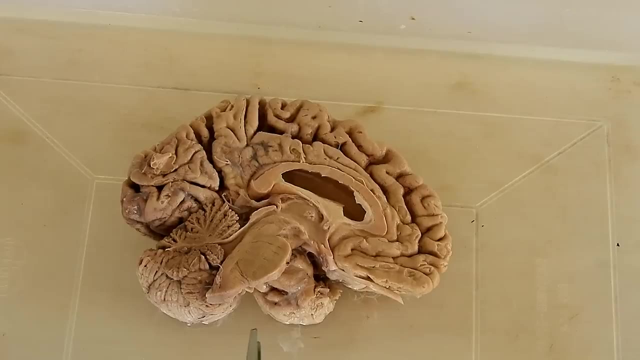 is again divided into two parts: The telencephalon, that is made up of a cerebrum, and a diencephalon, that is mainly made up of a thalamus and the hypothalamus. The midbrain is connecting the forebrain to the hindbrain. 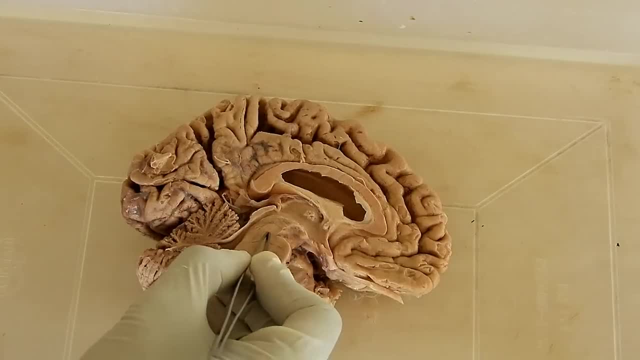 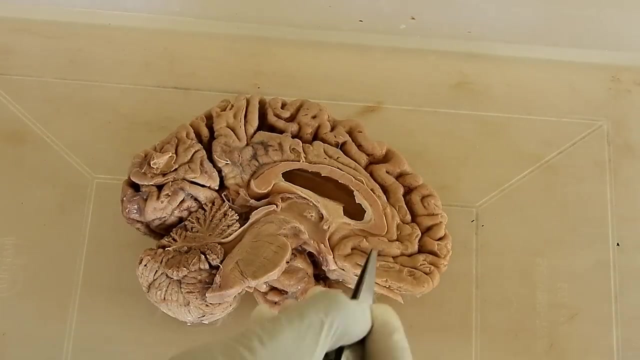 And the hindbrain is made up of, anteriorly pons in the medulla and posteriorly with the cerebellum. Now we discuss the structure seen in the mid-sagittal section of a brain. First we see the structure seen in the cerebral hemisphere, on the medial surface of the cerebral. 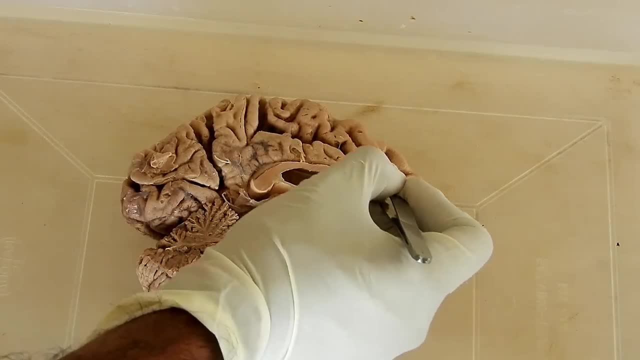 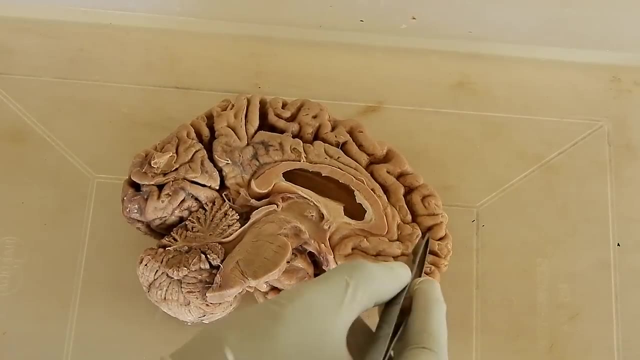 hemisphere You can see the depressed area which is known as the sulci, and in between the sulci There is a gyrus, The main sulci on the medial surface of the cerebrum, in the mid-sagittal section. here you can see the c-shaped sulci in the upper part. 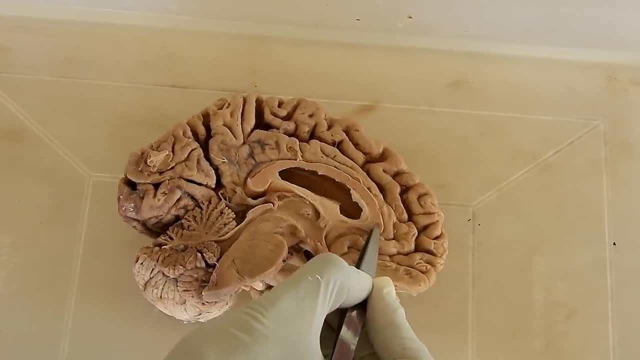 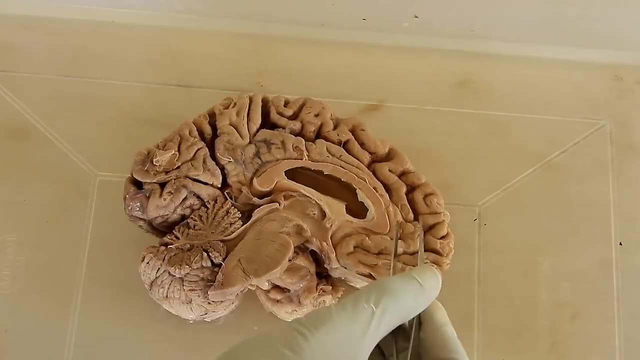 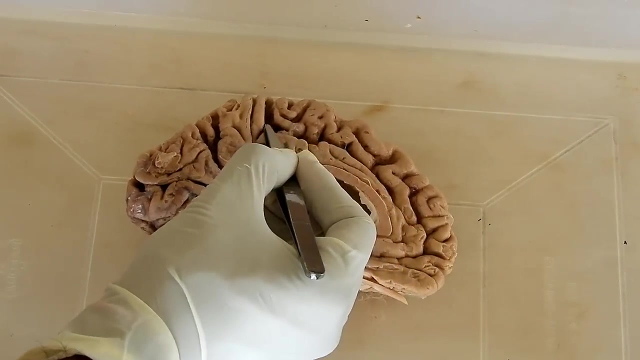 That arch is above this cut arch fiber. this cut arch fiber is a corpus callosum. Just above it there is a arch sulcus which will start anteriorly to the corpus callosum and callosum and it will ends just above the posterior end of the corpus callosum. it will arch up fast. 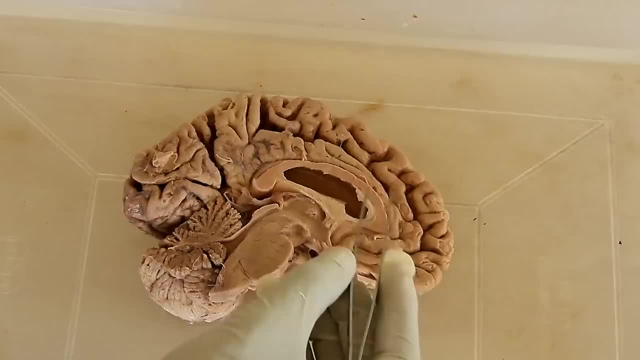 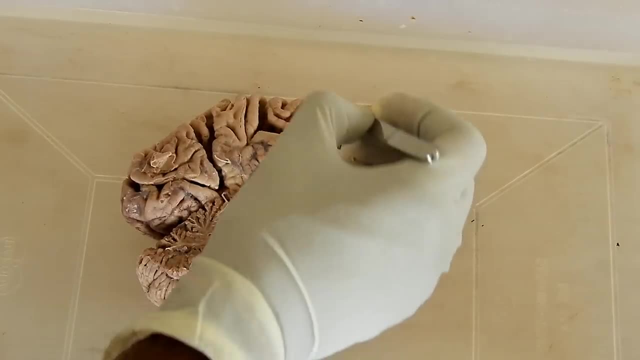 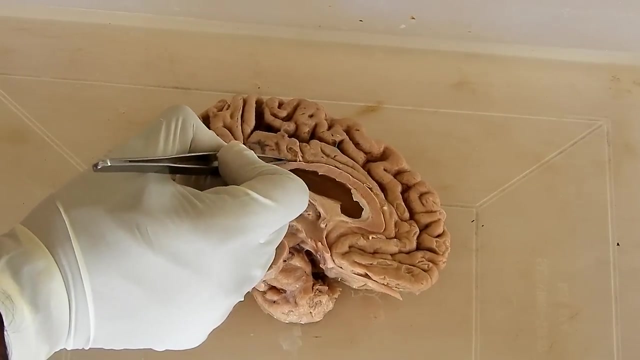 this is known as a cingulate sulcus. now, just below the cingulate sulcus, there is a cingulate gyrus which is separated: separates the corpus callosum from the cingulate sulcus. now, the cingulate gyrus is separated from the corpus callosum by a callosal sulcus. okay, now in the 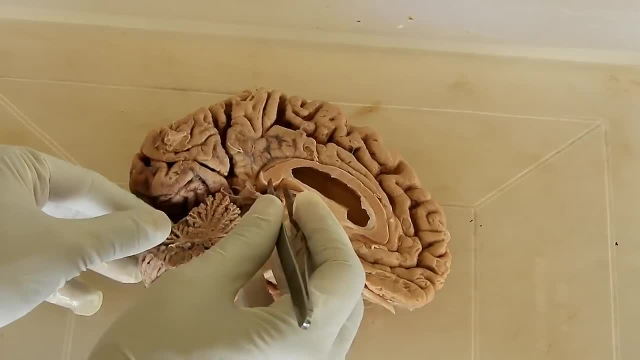 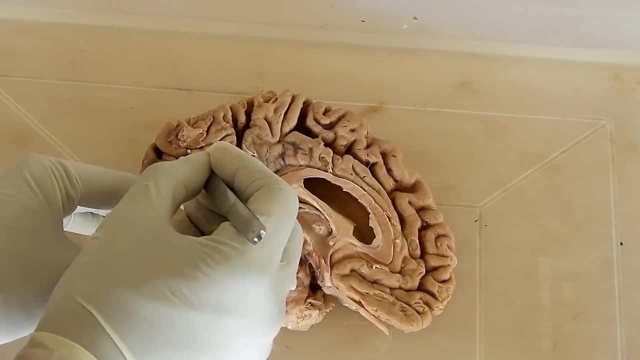 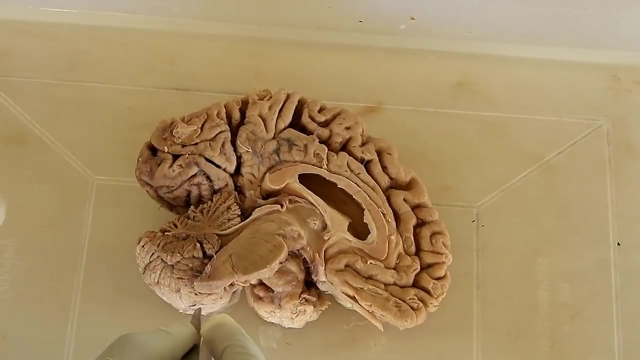 posterior part, the one sulcus which start just below and behind the posterior end of a corpus callosum, and it is going backwards, with the convexities facing upward. this is known as a calcareous sulcus. okay, now next, from the middle of the calcareous sulcus, one or another sulcus will 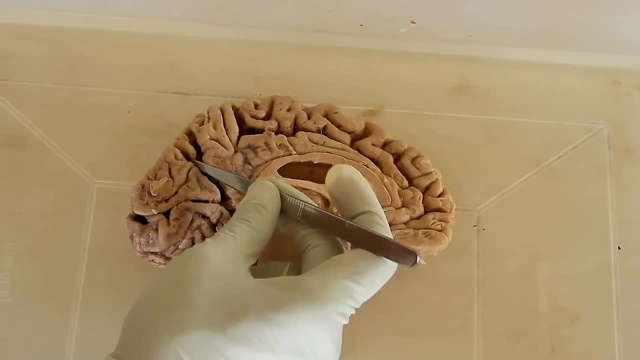 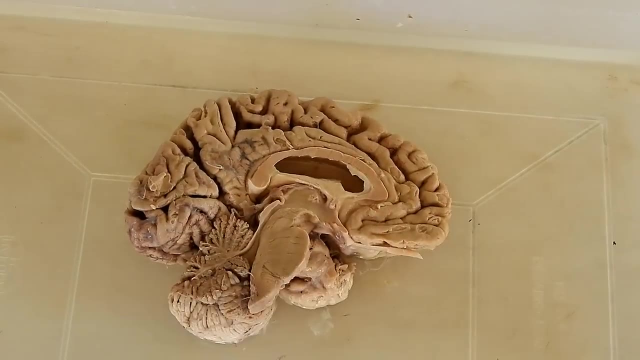 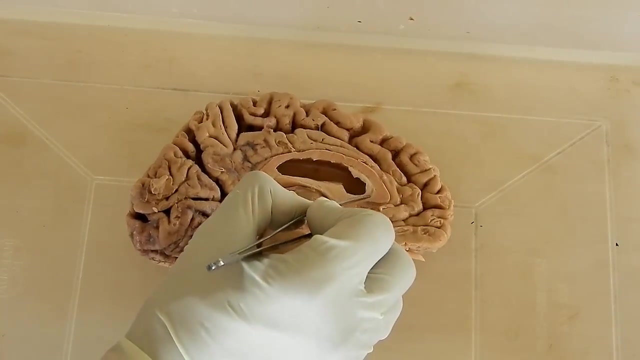 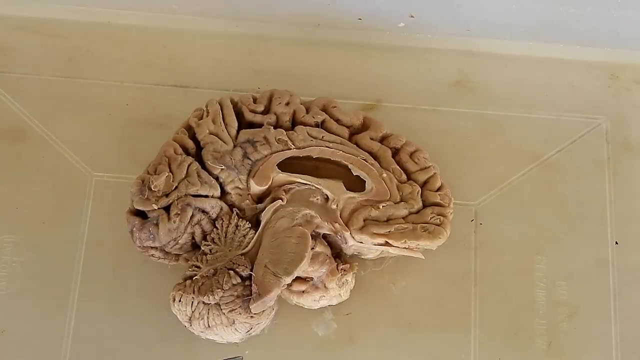 arise which going backwards and upwards, which is known as a parieto-occipital sulcus. so these are the sulci of a medial surface of the cerebrum. now here you can see the cut part of a c-shaped structure. this is a corpus callosum. now, the corpus callosum are the: 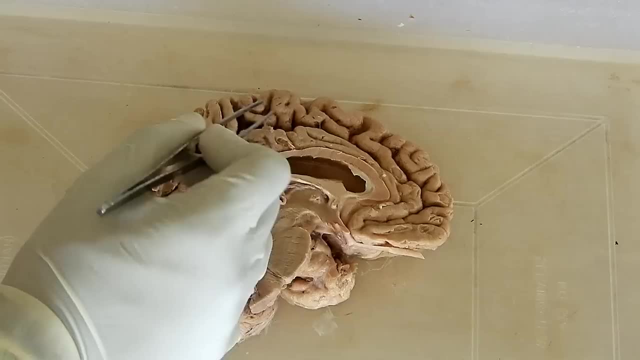 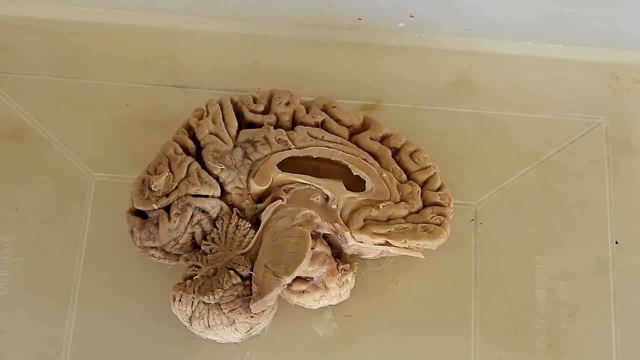 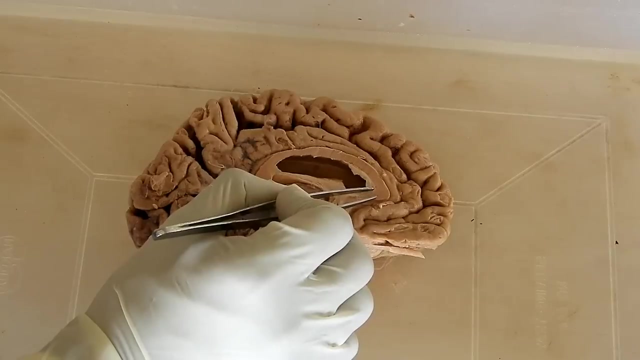 commissural type of a white fiber which interconnect the different lobes of the two cerebral hemisphere. the corpus callosum is having the four part. the anterior most part is known as a genu. from the genu arises the thin bundle of the fiber which is going. 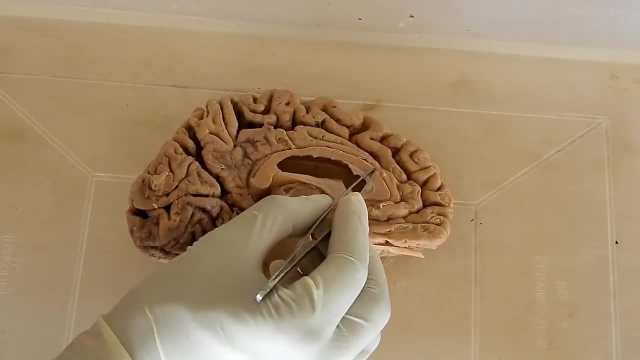 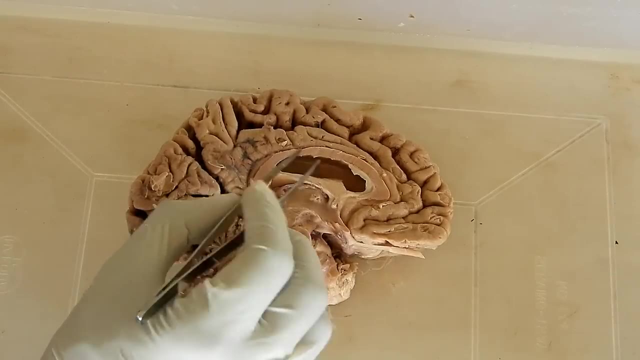 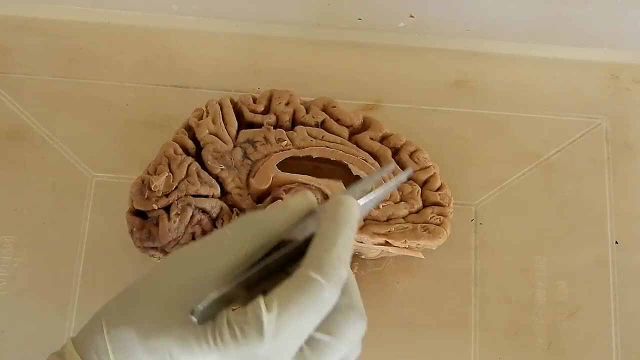 backwards and the downward, which is known as a rostrum. the middle main part is known as a body or trunk of the corpus callosum and the last massive part, posterior extremity, is known as a splenium of a corpus callosum. now, below the corpus callosum, you can see the cavity which is known as. 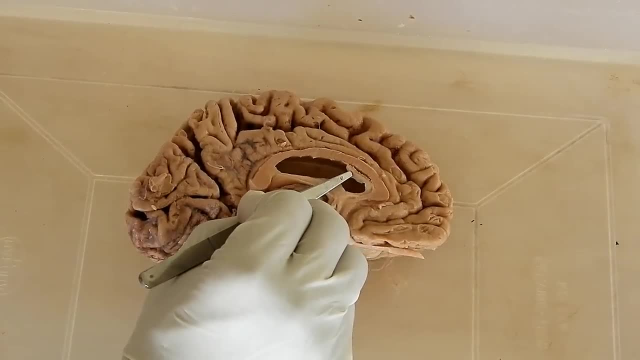 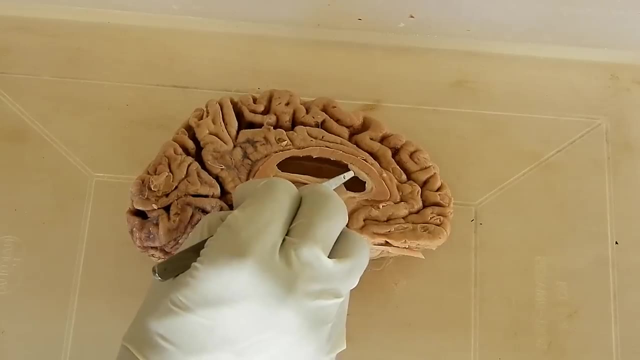 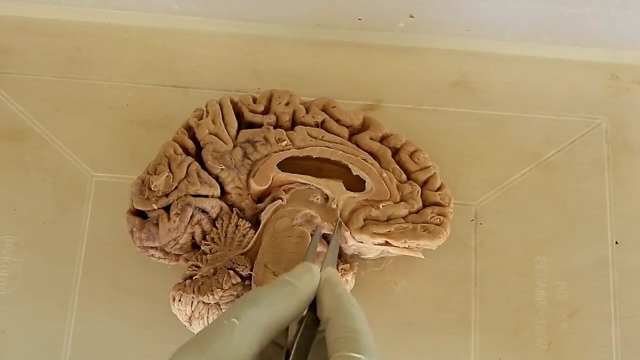 the third ventricle. now the two lateral ventricle are separated by one septum which is attached to the lower border, lower concave border, of a corpus callosum, which is known as a septum pellucidum. here you can see the part of the septum pellucidum. okay, now, below the corpus callosum and the 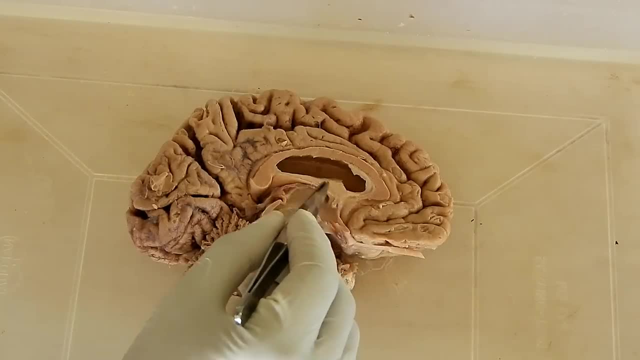 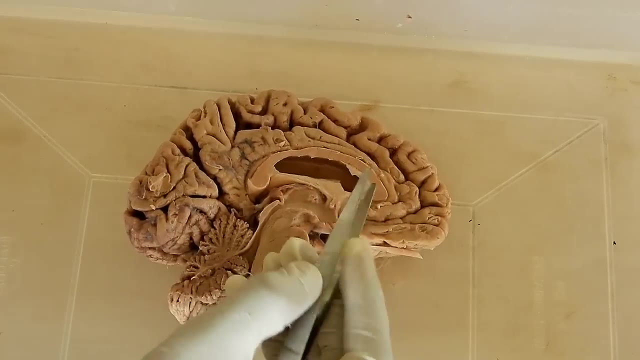 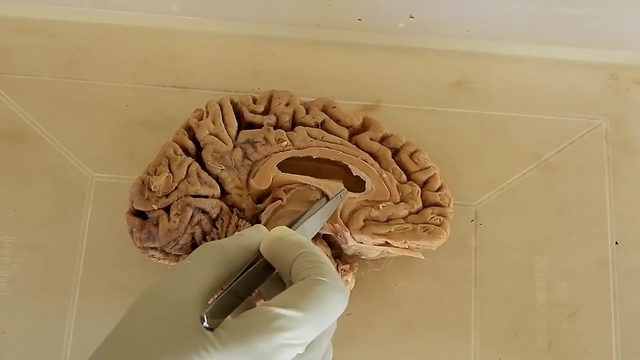 lateral ventricle, here the part of the diencephalon thalamus and the hypothalamus in which there is a exposed cavity of the third ventricle that we will discuss later on. the third ventricle is connected with third ventricle through this foramen, which is known as. 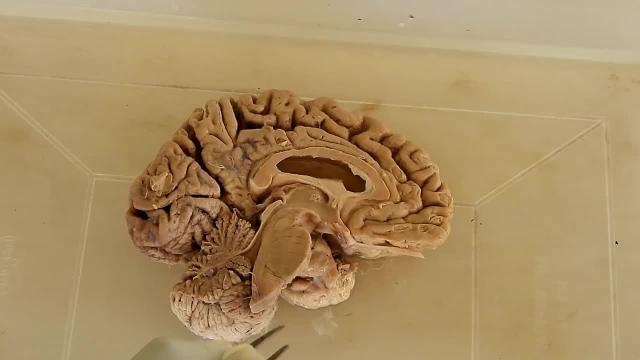 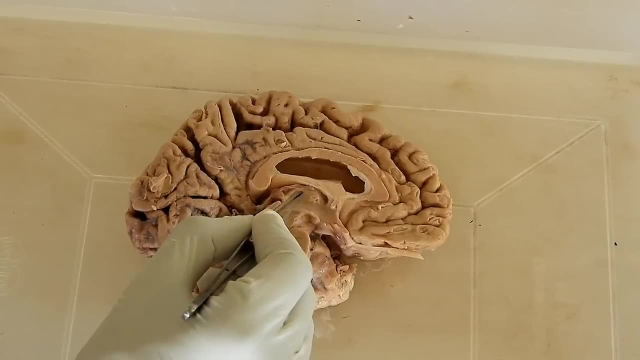 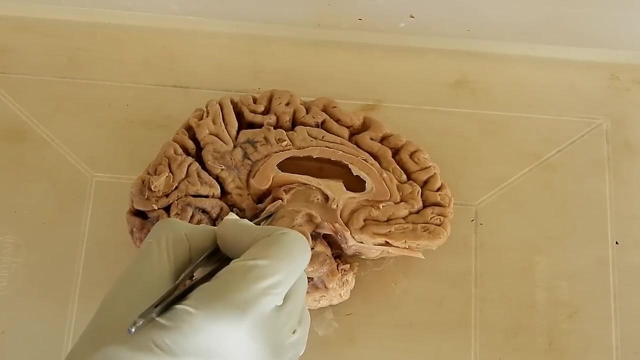 interventricular foramen or foramen of munro. now we going backwards and downwards. this part is a made brain. the cavity of the third ventricle is continuous with the cavity of the mid brain, which is known as a cerebral aqueduct, and cerebral aqueduct below it is continuous or communicating. 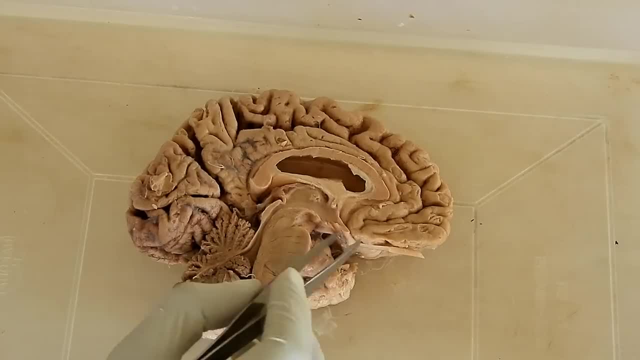 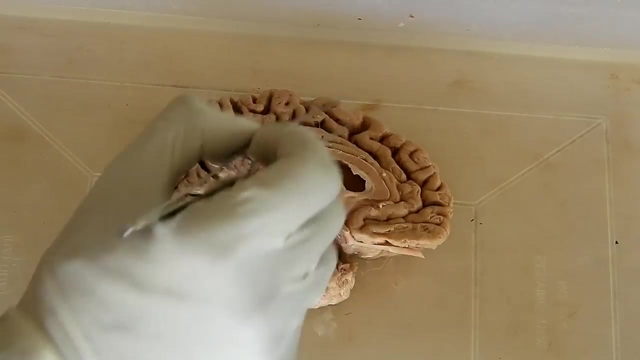 with the cavity of the third ventricle, the fourth ventricle, which lies between the pons and the medulla, in front and the cerebellum behind. so in the, this three, this uh different part of the brain, lies the different cavity. in the talencephalon lies the cavity of lateral ventricle. between the two diencephalon lies the third. 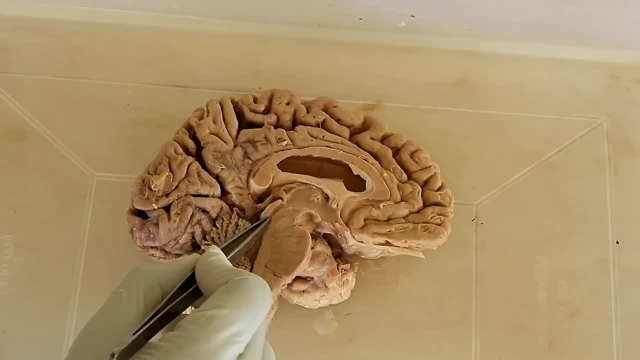 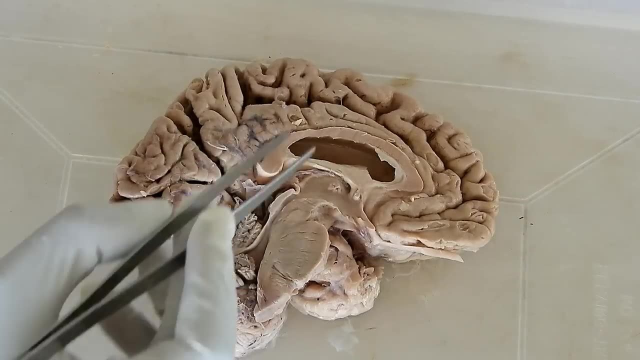 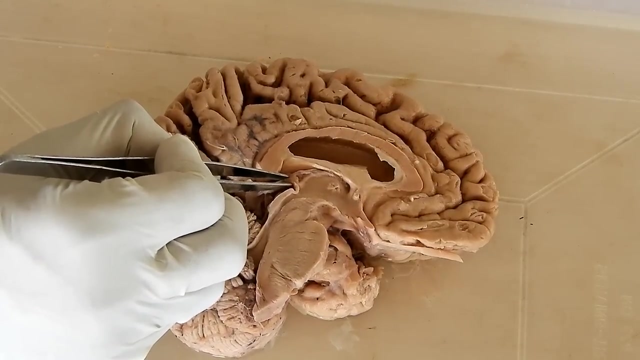 ventricle, in the midbrain lies the cerebral aqueduct and the hindbrain lies the fourth ventricle. now the other structure you can see in the sagittal section, here in relation to the third ventricle, posteriorly you can see this small body. this is called a pineal gland or a pineal. 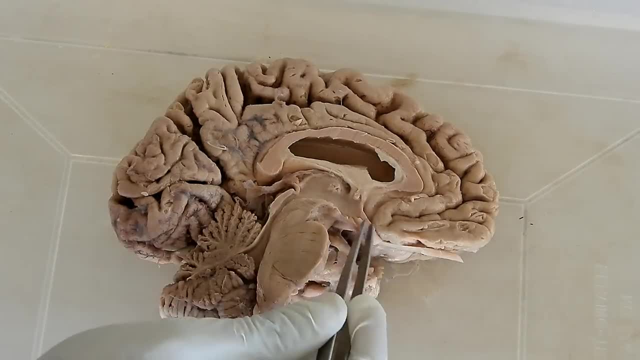 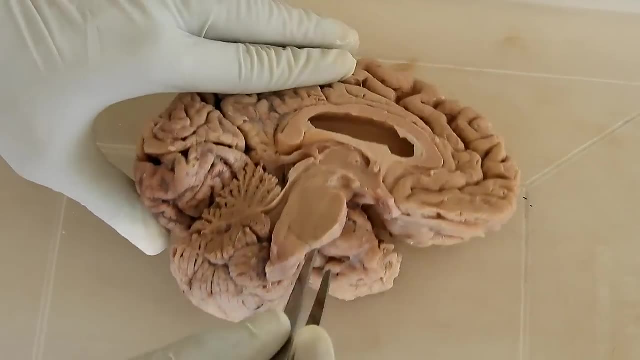 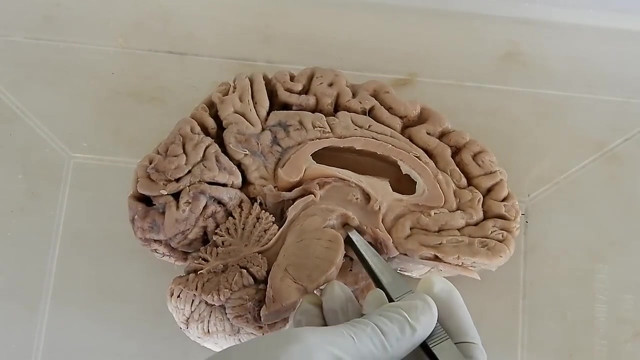 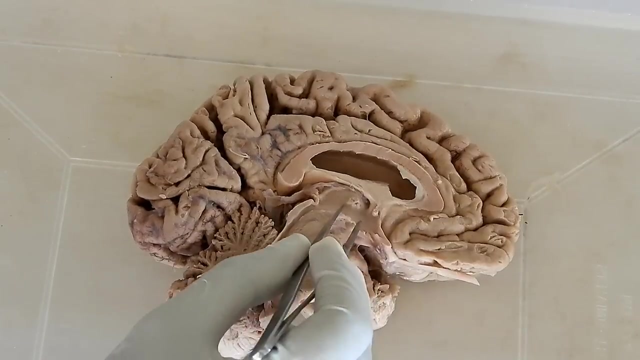 body. now, here, anteriorly, you can see the rounded structure in the lower part, in the base of the brain. this is the mammillary body. now, behind the mammillary body, you can see the part of the midbrain, here medially, the crust cerebri, and this one is a tegmentum of a midbrain. this will constitute 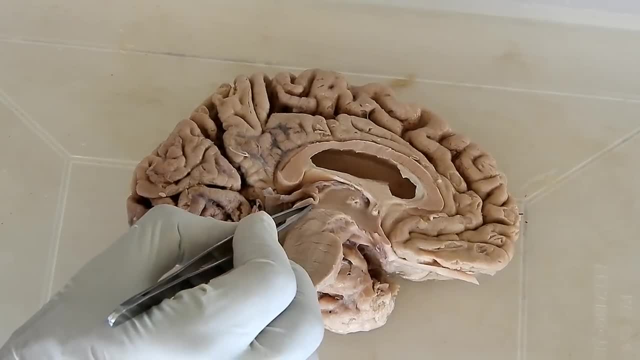 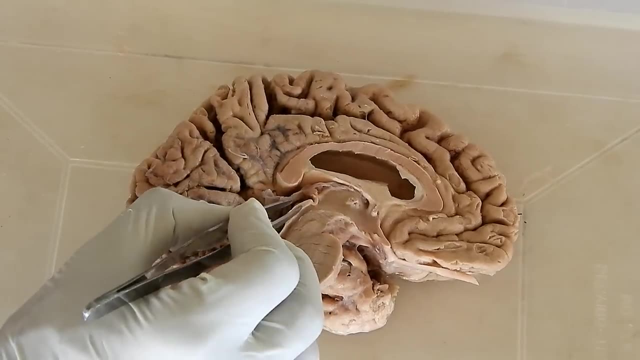 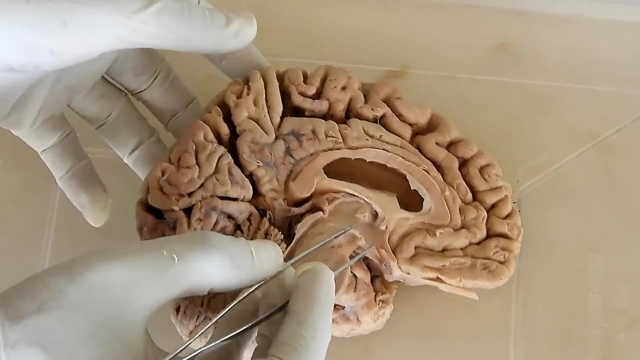 the cerebral peduncle. now behind it there is a narrow cavity which is known as a cerebral aqueduct, and behind it the part of the midbrain is known as a tectum of a midbrain. now, in the posterior most part of a midbrain, you can see the two oval swelling, the superior. 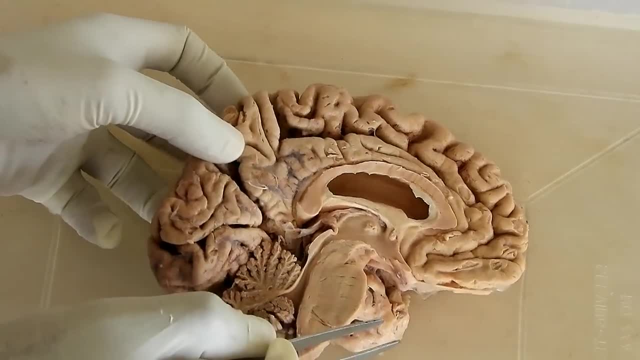 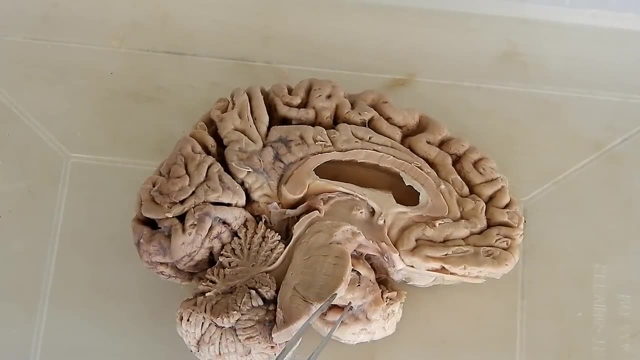 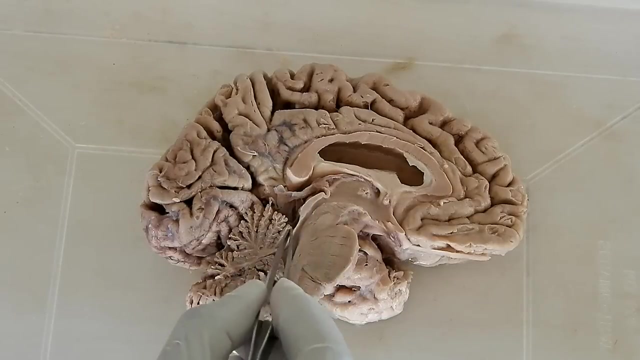 and the inferior colliculus of a midbrain. right now, below the midbrain, there is the midbrain below the midbrain. this part is a pons and this is a medulla. now, here you can see the cerebral aqueduct below. it is communicate with the cavity of the fourth ventricle, which is a tentacy having. 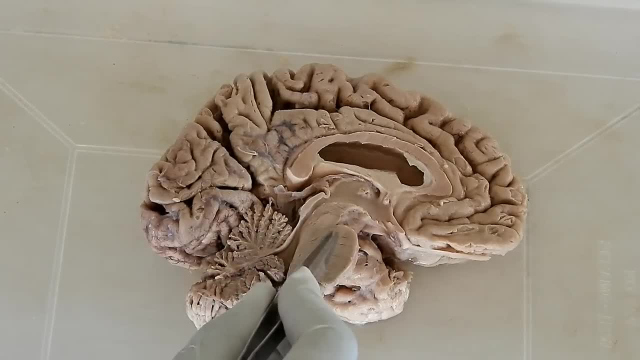 the floor which is facing anteriorly, which is formed by the posterior surface of the pons and the posterior surface of the upper part of the medulla oblongata, whereas the roof of the fourth ventricle is directed posteriorly, it will indent going into the white core of a cerebellum. now, this white core of the cerebellum,